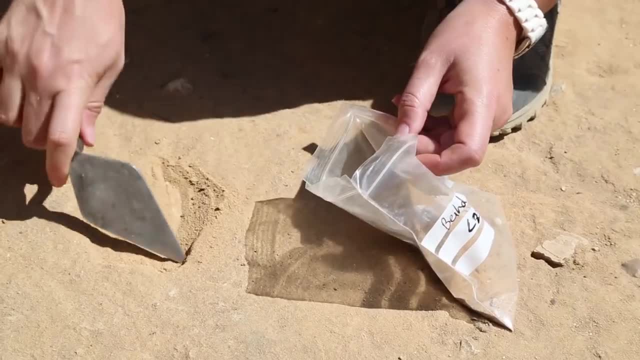 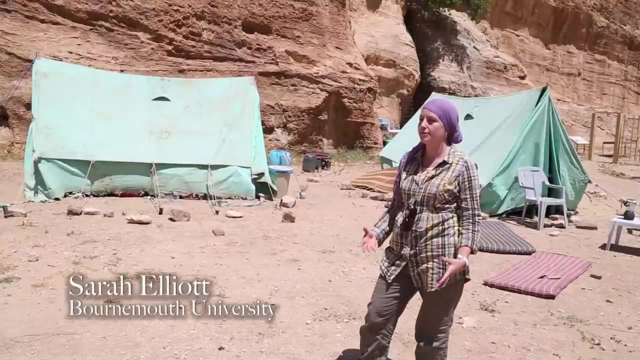 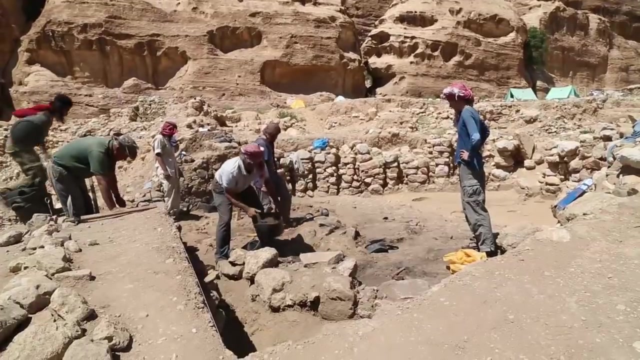 about the one thing. It's about what it means as a whole. So, on excavations, often you live very close to the site. So, for example, at this site they have tents and they sleep here at night and they walk just over to the site, which is very close. 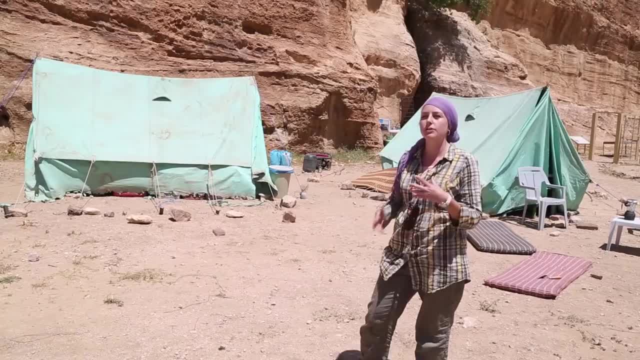 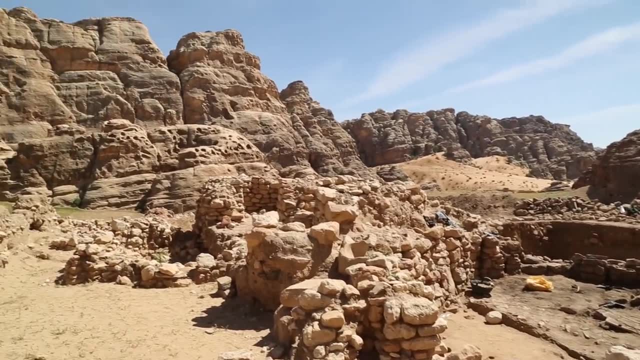 And you live with a team. You have to get on with everyone. Everyone chips in, You make food, You sleep here And you have amazing stars at night. the scenery, the whole sort of being outdoors and sort of roughing it a little bit, It kind of adds to the excitement. 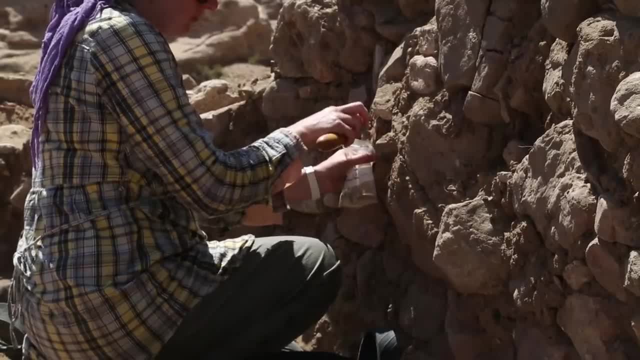 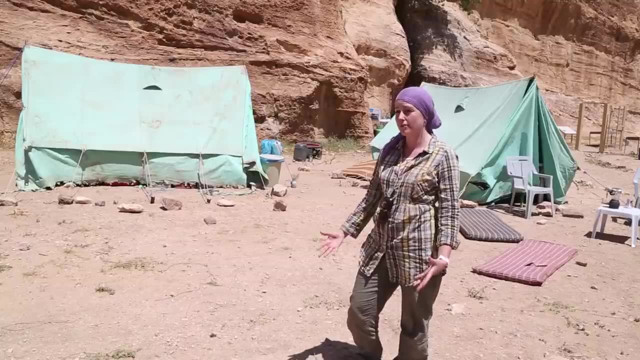 of the job. So I first started getting interested into archaeology When I was 11, and I visited the pyramids in Egypt And then I went on to do it as an undergraduate at university, went on to do a master's, been on many excavations and really 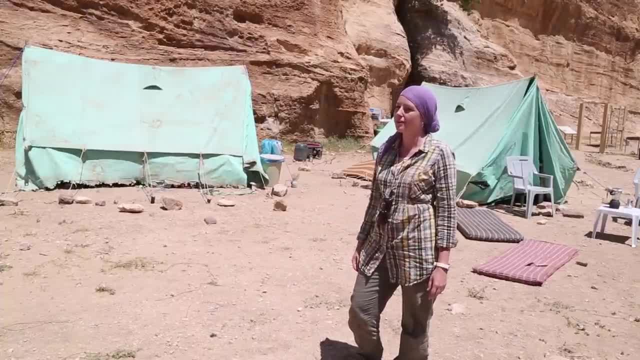 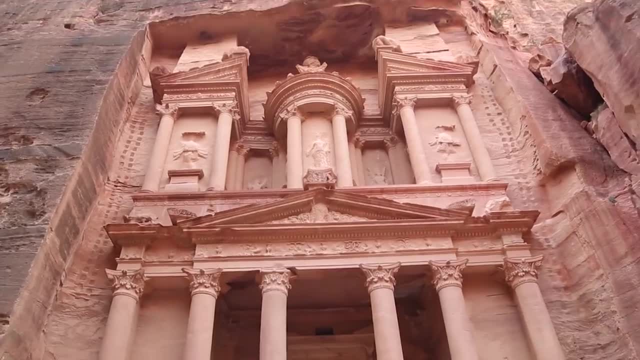 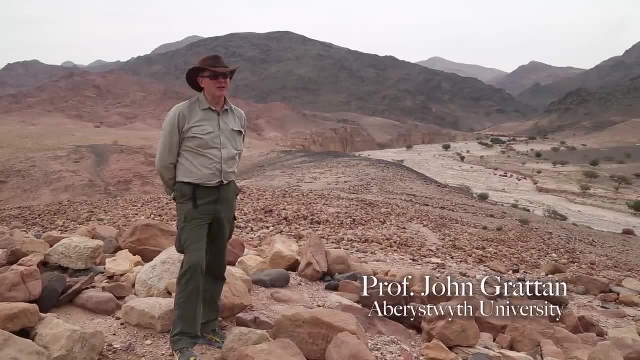 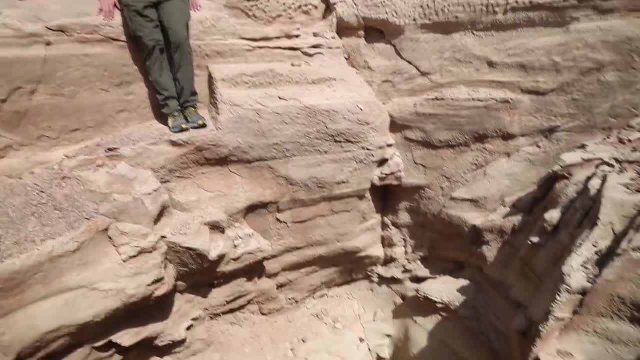 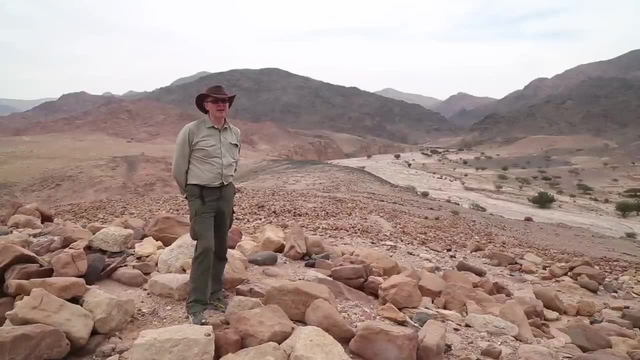 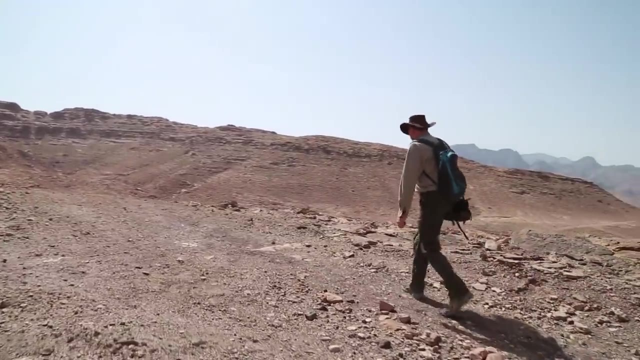 and the interaction people have had with them through that period of time. If you do an archaeology degree, you're tackling very big and complex problems. So here in Wadi Feinan we're dealing with a very complex problem, which is: how do people survive here? 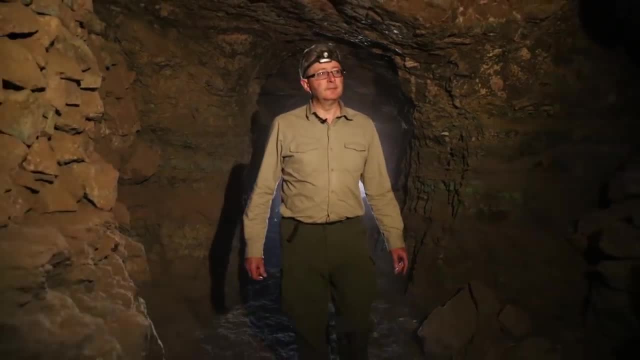 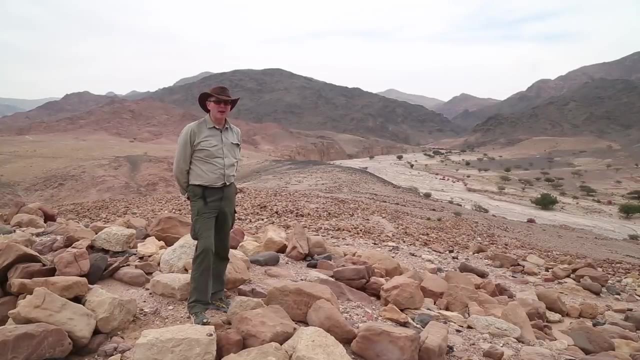 over 8,000 years years. how did they develop the first factories? how did they run a massive copper mining and smelting enterprise to do that? so you have to bring together an enormous range of skills and tools to do that. from remote sensing imagery: 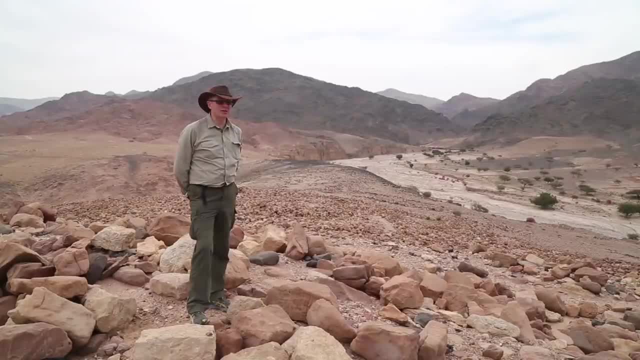 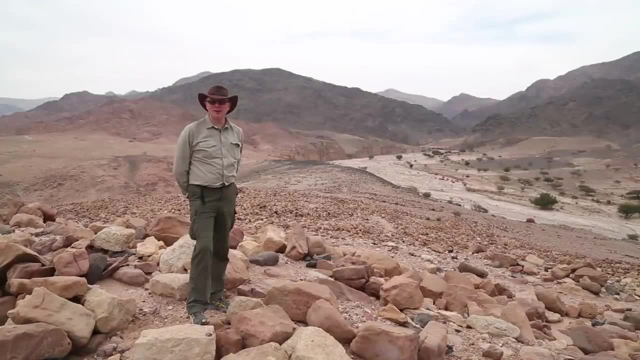 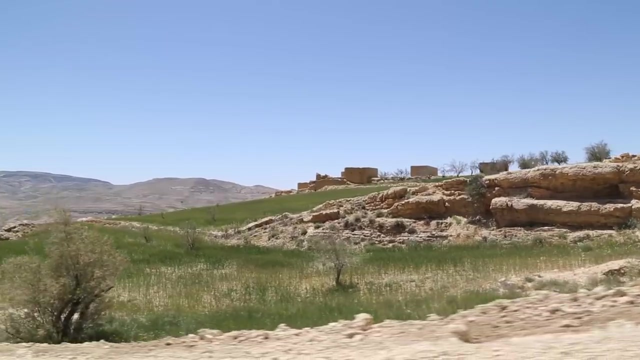 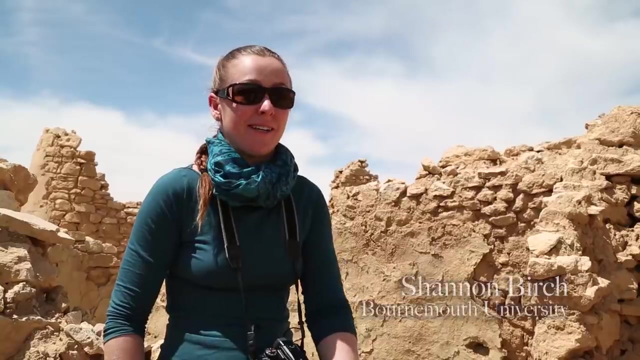 satellite input, satellite imagery from space, soil science, technical science in in laboratories, mathematics, statistics. so actually, rather than archaeology, be in the vehicle that you're developing a whole range of really key graduate skills. today we are creating a photo log of the entire site, so that basically means we 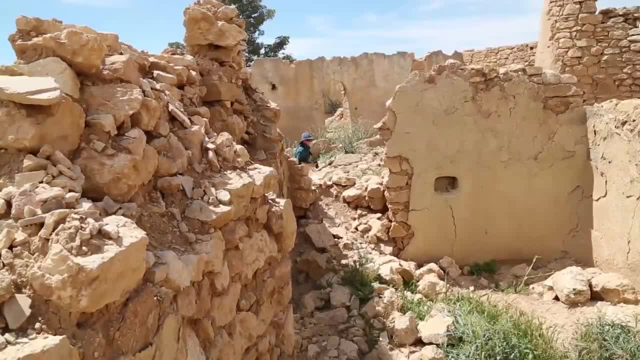 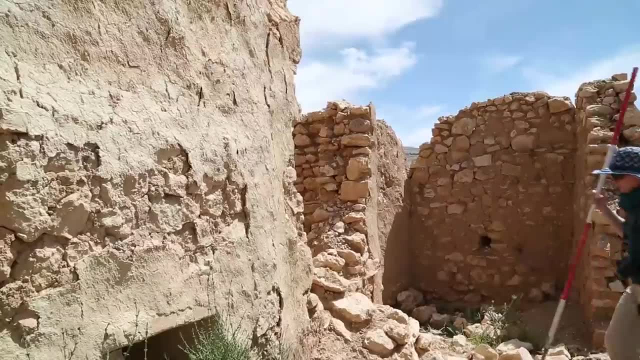 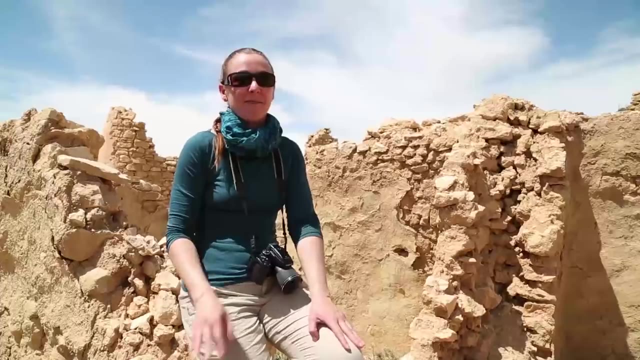 go around to each building. we photograph the whole building generally and then if there's any specific aspects within that building that need photographing, like a particular niche or a platform or a hearth, we photograph that individually as well. the nice part about this project is that we're creating a little bit of 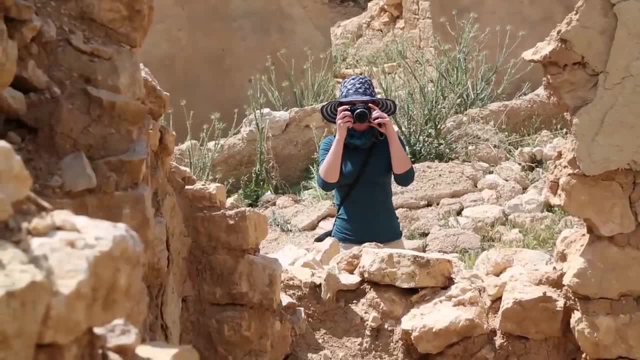 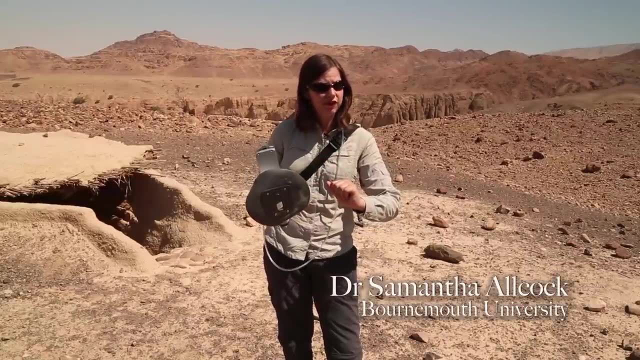 history for everybody to use you. this is a portable XRF scanning device, and what this does is it sends out x-ray beams from the front of the instrument and into whatever we've decided we're going to be scanning, and it will collect those x-ray beams back. 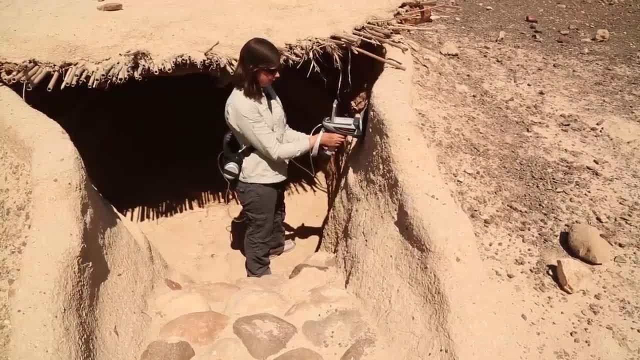 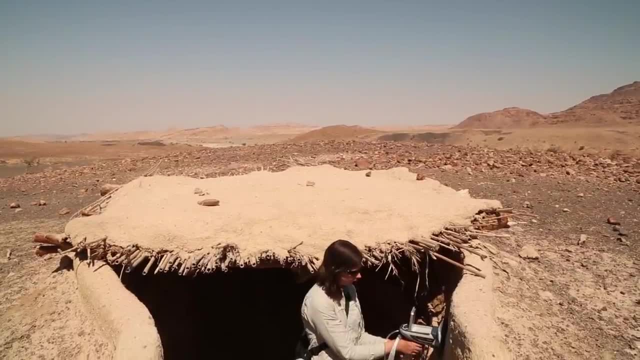 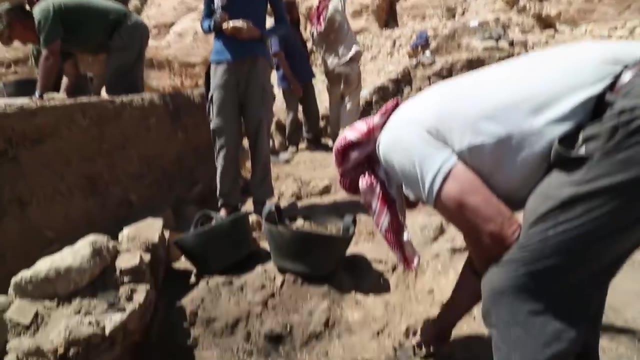 and let us know what elements are within the substance we are scanning. you don't just learn about past societies and cultural development. you learn other skills. so IT is quite a big components of an archaeological degree come from a range of backgrounds. Geography is one of these backgrounds, an environmental 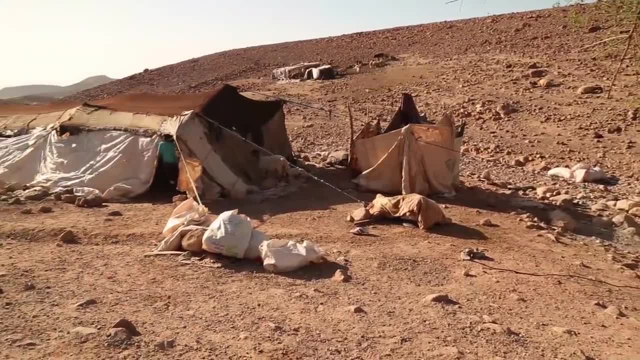 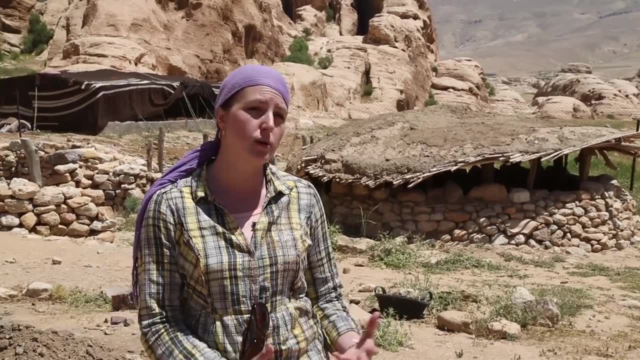 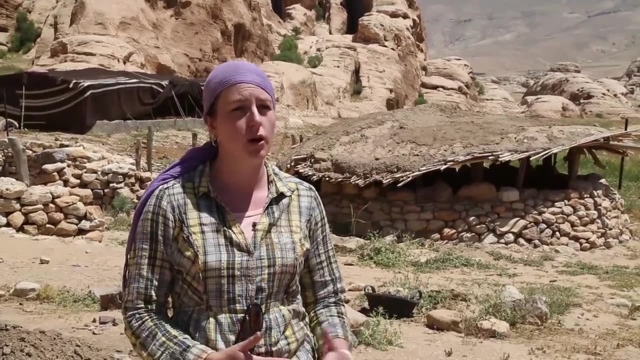 background or perhaps something like a history background and how people develop. I applied to do archaeology at university. I had biology, history and geography, but only because they didn't offer archaeology where I did my A levels. But it's more the grades depending on what university you go to, and it does really range. 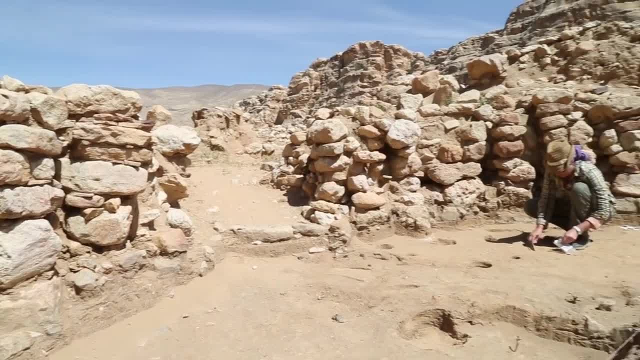 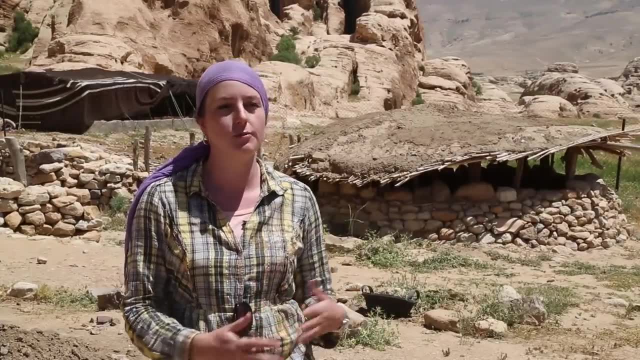 but you don't need to have a specific background, just A levels, to go on to university. So people can come from an art background and do archaeology or a politics background and I try to do subjects which might be more relevant, but it's not necessary. 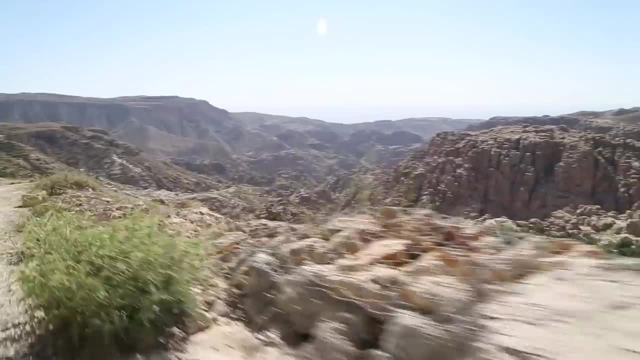 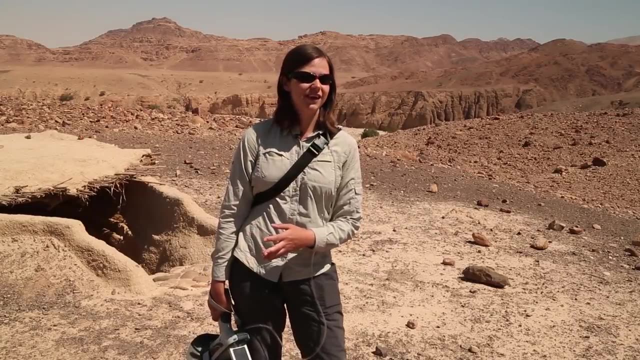 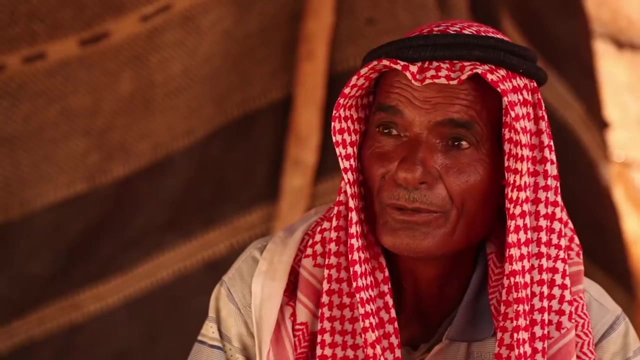 You never get to travel the world normally as a young person, but as an archaeologist you can come out to these different sites and experience different cultures, different environments and different countries, and you get a much more broad perspective of life. I feel proud.